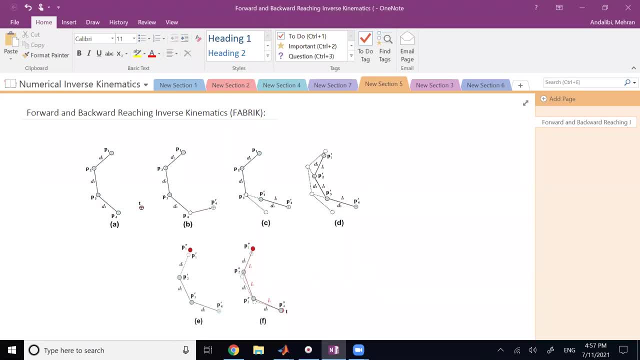 Hello everyone, In this video we are going to talk about another method for numerical solution of inverse kinematics problems and that is called forward and backward reaching inverse kinematics or fabric, which is an interesting heuristic method, And let me explain that again through an example to you. So here again, assume that we have the three degree of freedom: planar arm, which is pinned down at point P1,. okay, 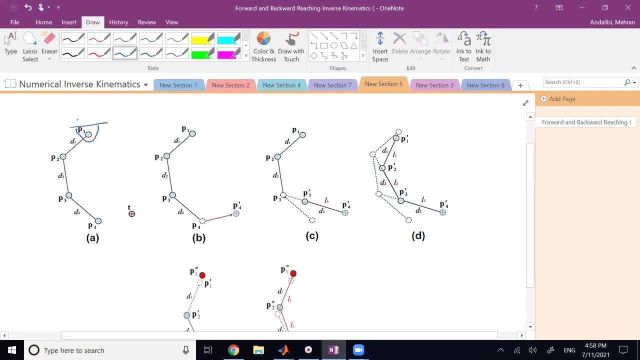 So here at P1, you have a pin. It is not supposed to move from that pin, ideally right. That's a rigid pin. This is my initial configuration of the pin. So I have the robot with some initial angles and now I ask the robot to go to this point T, the target point. 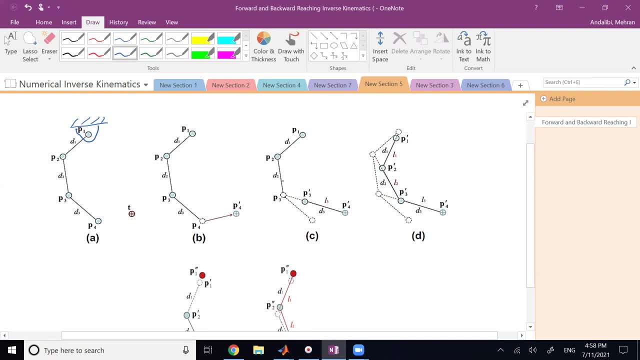 Well, this is the way we go about it. We go first in a forward manner and then backward. What does that mean? In the forward stage, this is what we do: First, we try to put the end effector, which is here at point P4.. 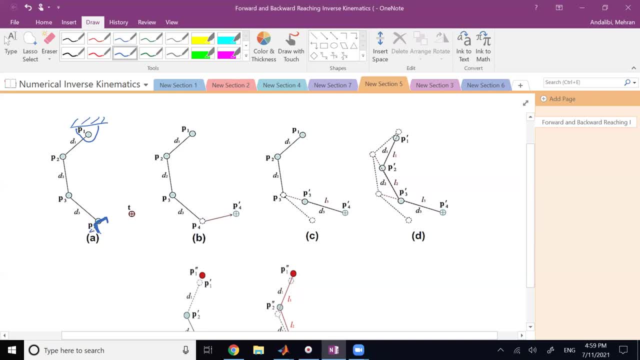 We try to move the end effector at P4.. We try to move the end effector at P4.. We try to move the end effector at P4. We try to move it and put it right at the target, as if we could get it solved in just one single step right. 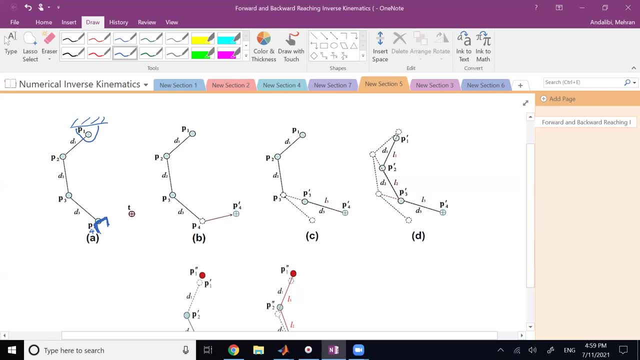 So we put P4 right at the target. So P4 now comes to this new point called P4, prime, which is the same as the target. Good, Now what happens here is, if point P3 does not move, then the length of this member, which here we show, be D3, it has to be longer, It has to be now this much. 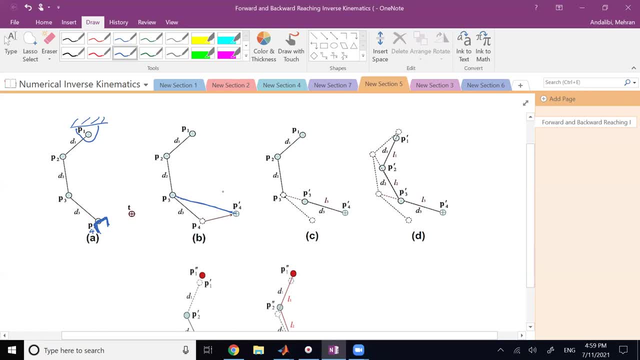 And this cannot happen because we here assume that this member is a rigid member and this joint is a rotary joint, not a prismatic joint. We already rotated it right, And so this member now has to change its angle, from the line connecting P3 to P4 to now P3 to P4, prime. 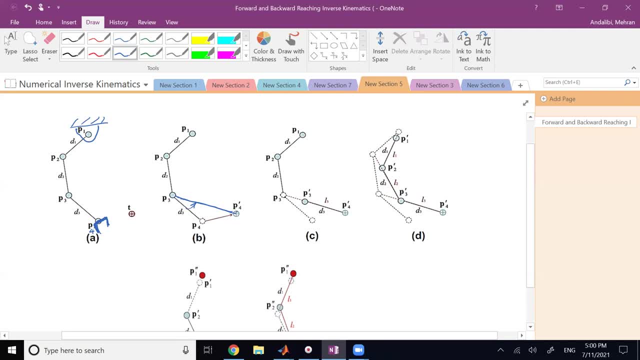 So we rotated the angle, but clearly we cannot stretch the angle The member. So if I want to keep the member to be the same size as what it used to be, this is what I do: I connect this point P4 prime, the new location of the end point P4, which is again the same as target. 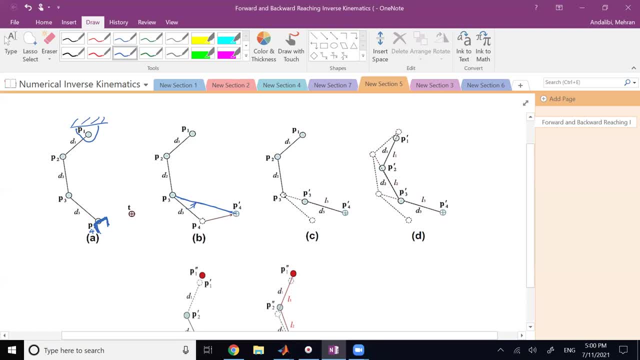 I connect it to the other end, P3. And then, along this line, I separate a distance from P3. And then, along this line, I separate a distance from P3. And then, along this line, I separate a distance from P4, prime. 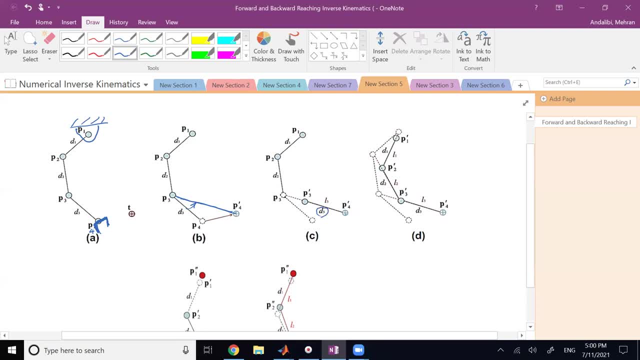 I separate a distance, the same as what? The same as the original length of the member, And that gives me point P3, prime, which is where point P3 should be if I do not want the member from 3 to 4 to be stretched. 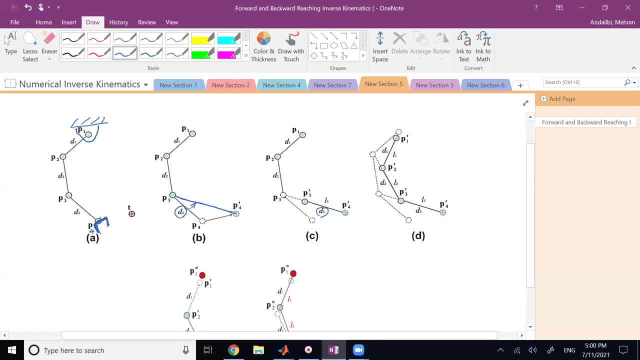 Good. So it's like I have transformed this member from here. now it is here, And if you look at this step, you see it's very similar to the CCD. In CCD we did the same thing. We focused on joint 3, because that's where the last rotation was. 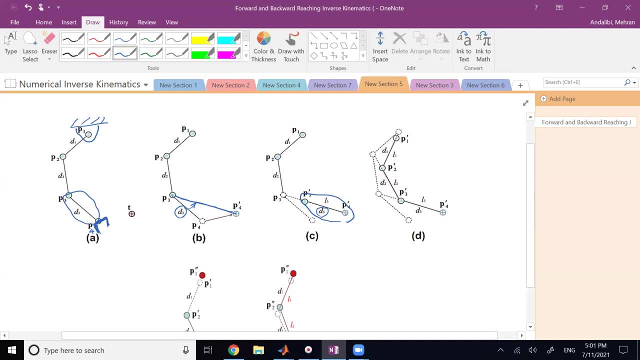 We focused on the last joint, We connected the target to that point And we tried to align the line going from joint 3 to the end effector to what With the line that goes from joint 3 to the target. So that's exactly what we did. 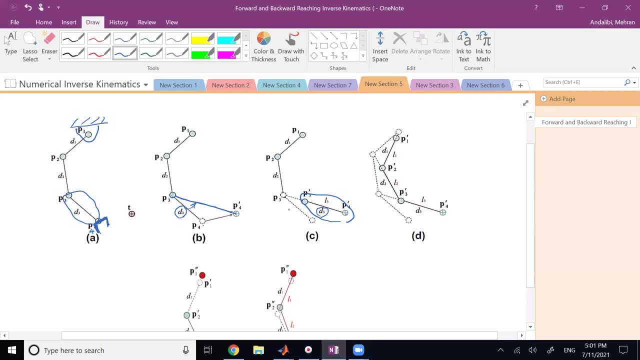 Last time we also aligned. But what's the difference between here and CCD is in CCD we did not move. at point P3. We kept it in the same location and therefore we could never reach the target point. We could come here. 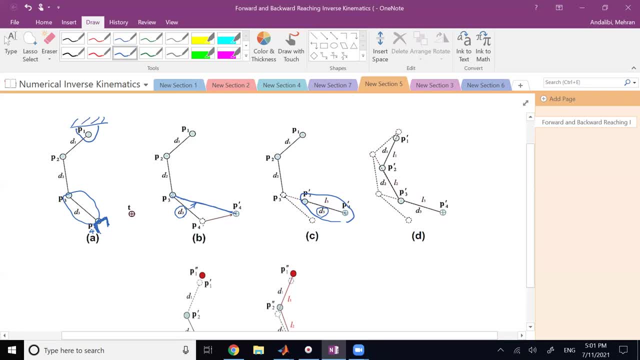 Instead of separating the distance from the end, we separated the distance from the beginning because we assume it cannot move, And so we end up here, if you remember, in CCD. So my member was this guy here in blue Instead of this guy here in red. 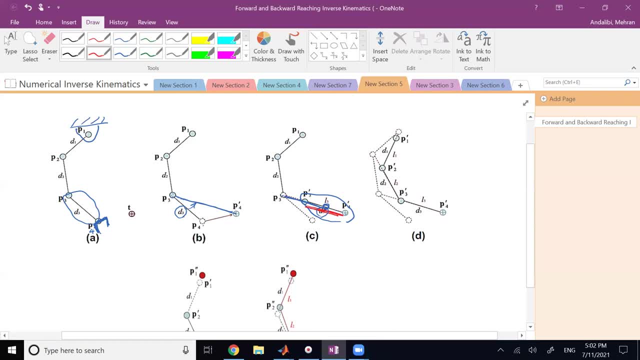 Right In CCD again, the joint was immobile, The endpoints could move. here We fixed the endpoints to the target and we moved the first point. Okay, So that's the difference. And now what does this one mean? 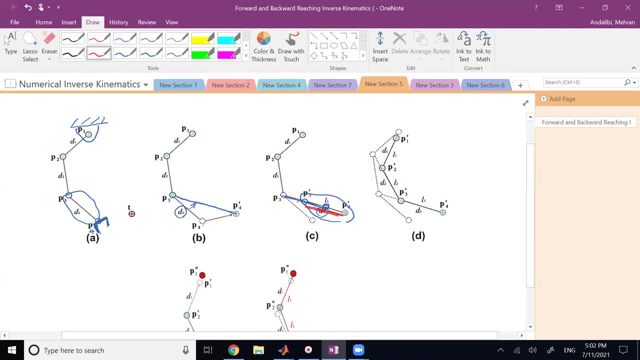 Well, fine, My P3 should come to P3 prime. Good, Fine, Now what Now if P3 prime is here again? if you look at the distance between P3 prime to P2, this length that is bigger than this D2.. 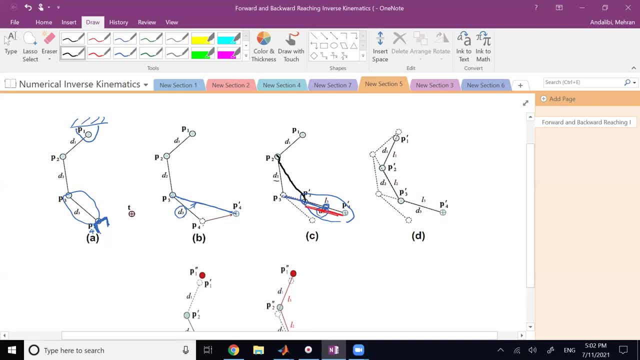 Right. So it means again, now the second member has to be stretched, which cannot happen because we only can rotate it. So what we do? we rotate it, We align the lines. So now The new coordinate, the new location, not the coordinate, the new location for P2 has to be aligned, this line which connects P3 prime to P2.. 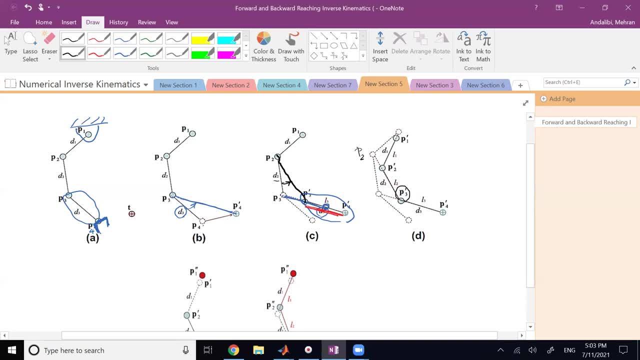 But again, since the length of the member cannot be stretched from P3 prime, I pick a distance of D2, L2 equal D2, from P3 prime And that gives me the new location of P2 prime. And then I go and connect P2 prime to P1. 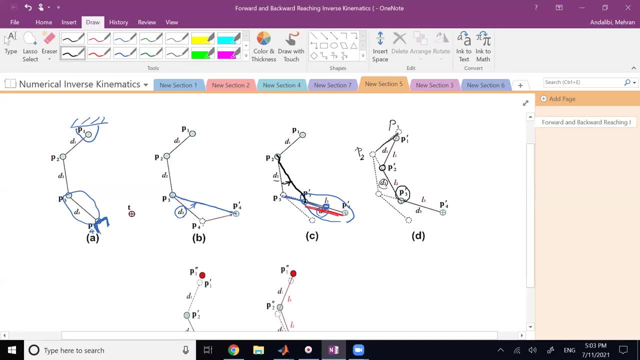 Clearly again, if you look, P1 to P2 is shorter than P1 to P2 prime. So what I do is again connect P2 prime to P1.. Then what Then? separate on this a distance of D1.. 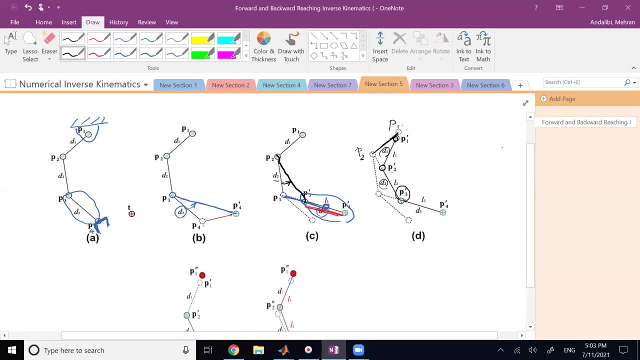 And that brings me to point P1- prime. So now, if you look, My robot can reach the target point, but something is violated. What The pinpoints? The pinpoints that was on P1, and it was supposed to be fixed point P1, is now shifted to point P1 prime. 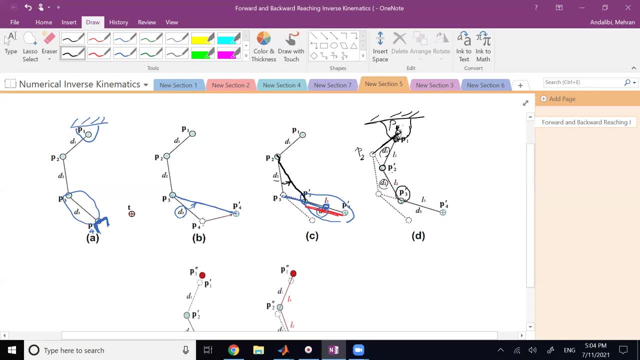 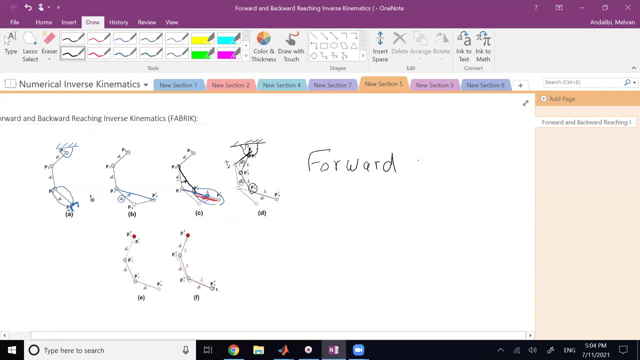 So the base support of the robot has moved and it cannot happen. This cannot happen. This is violating our physical constraints. So this stage, which we call the forward state, gets me, gets my end effect. So I can't go from the vector to the target, but it makes my ground support to mess up. 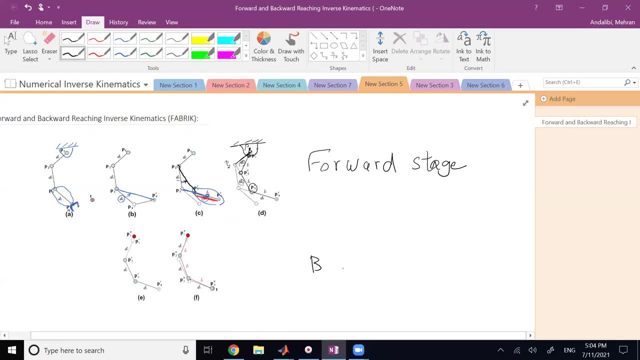 So we need to fix that in what we call a backward state. In this backward state we try to put the pin back. So we start with what we got from step number D- Here that's what it is- And say, well, I shifted my P prime from wherever it was. 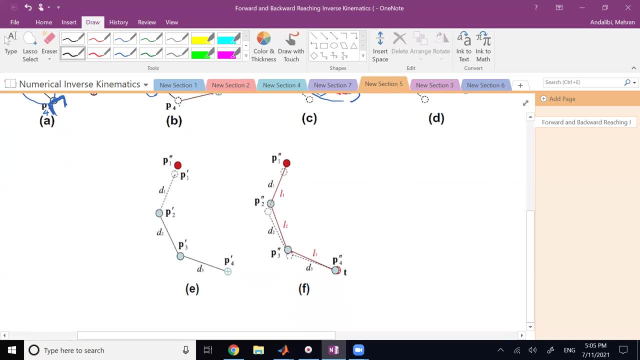 to this location. but that cannot happen. So let me go and put it back. How So I connect my P2 prime to point P? this P1 double prime is the same as original P1.. It's the same as the pinpoint. 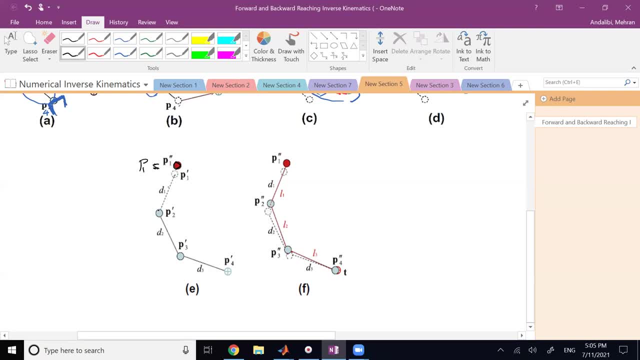 Let's go put it back. But again, since this member with length D1 cannot be stretched, so I connect my P2 prime to this new point, P1 double prime, which happens to be the same as P1.. I connect them. and again, on this line, 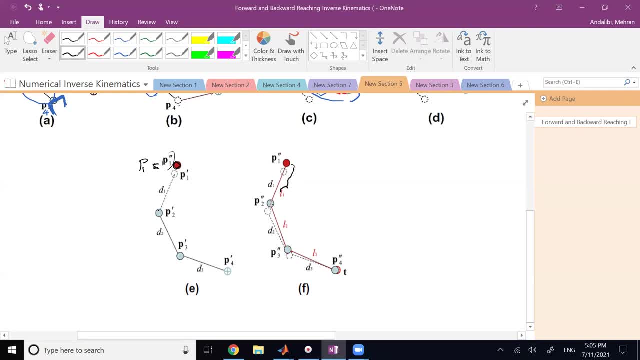 I'm gonna choose this distance correct. The same as what? The same as actual physical distance, And that means move the point P2 prime, which was here, So now this new point P2 double prime, And again that causes the next member. 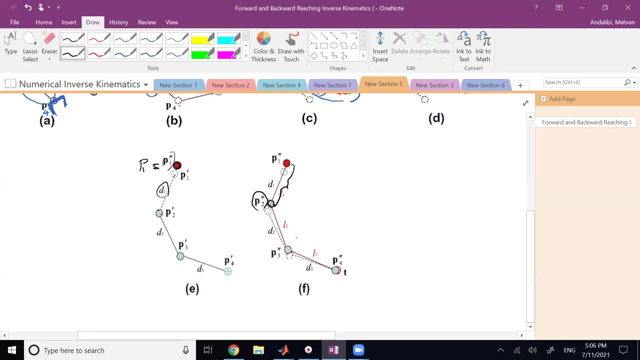 to be stretched, which cannot happen. So now what? Now I will connect my point P2 double prime to the P3 prime which is here connected, And then on that line, I pick this distance equal to D2.. That bring me down to P3 double prime. 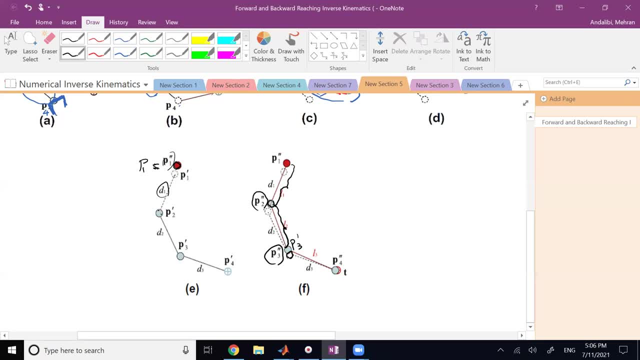 I connect my P3 double prime to the location I want And I connect my point P3 double prime to the location I want to the point P4 prime which is here in this red location. Again, separate the distance here: equal to L3, equal to D3.. 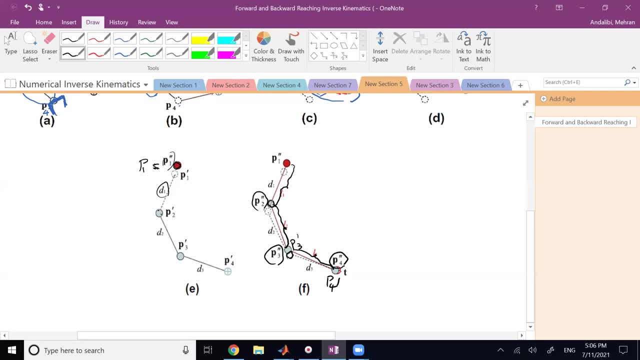 And that brings me to point P4, double prime, which is close to the targets, but not exactly now at the targets, But I could put the pin back, Okay. So in the forward stage it means put the end effector at the target. 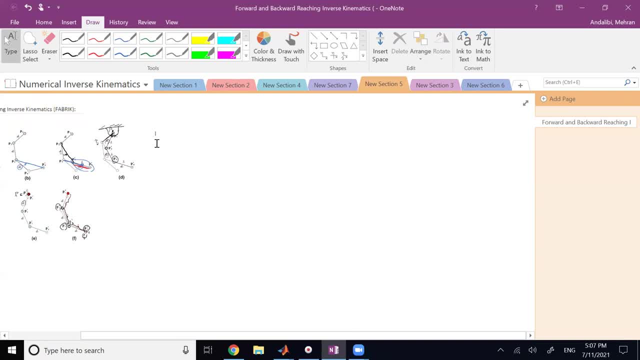 It's gonna be cleaner than write it here. So in the forward stage, it means putting the end effector at the target and modifying the locations of the joints Accordingly. by keeping the length of measurement, it's actually going to more or less do the same. 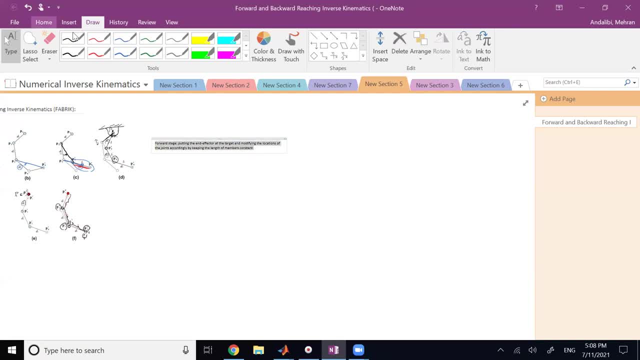 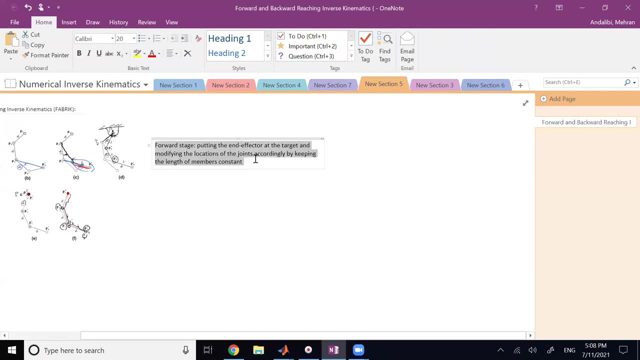 So the second thing again is the forward stage. So this is what you can describe as the forward stage. You can see it, the failure state is going to be the impact point And this is going to be the input point. So 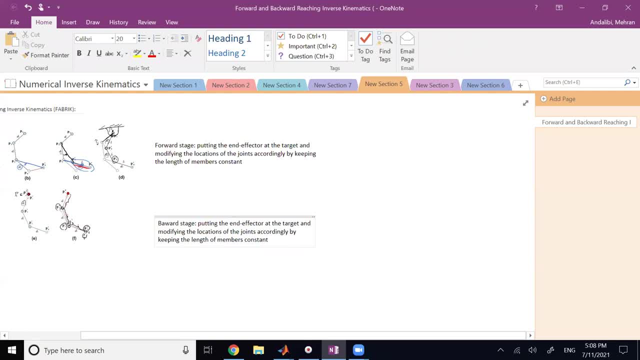 in the forward state. it's going to be the input point. It's going to be the input point. So now we're going to have to adjust the end effector, So this is going to be a little bit lower. This is going to be the input point level. 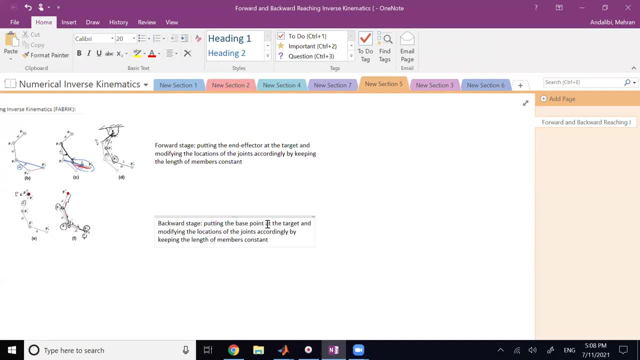 You can see, you can see over here, point back to where it was and modifying the locations of joints again accordingly by keeping the length of the member constant. So in the backward stage your end effector is not going to end up at the target point, at the very. 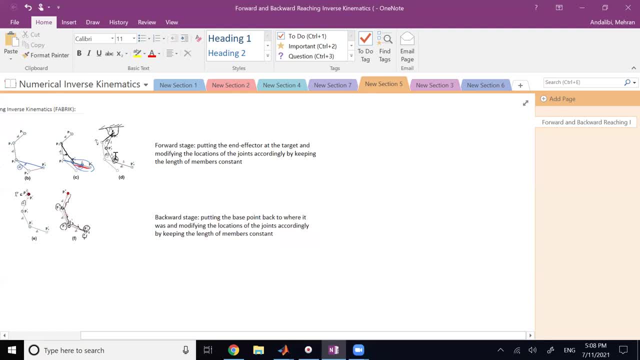 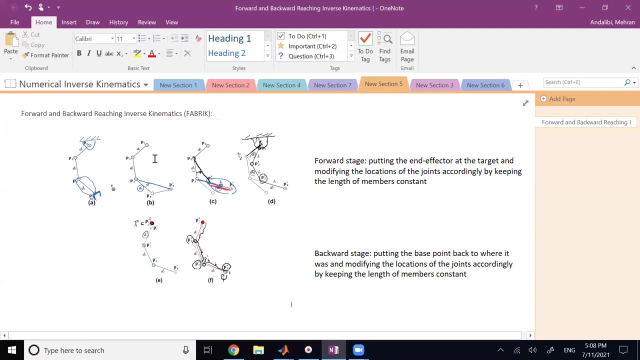 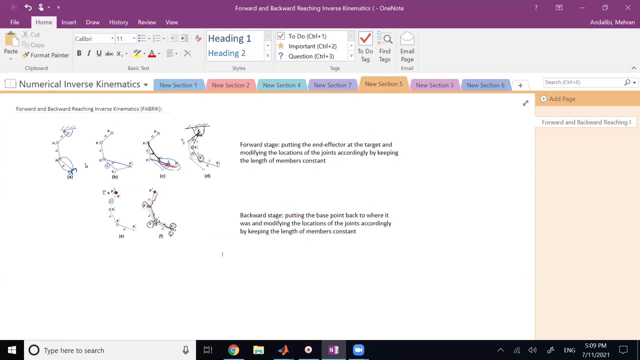 end of it. It's going to be closed, but at least you have not violated any- what Any? physical constraints. So with one step going through forward and then backward stage, you can go from being off to what To being very, very close. And if 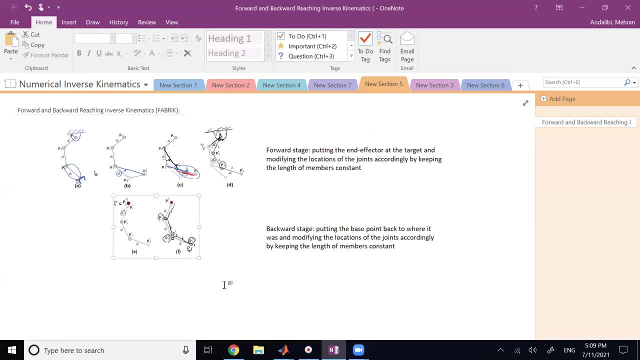 you repeat this forward and backward stage a couple of more times. you should be able to what? To get the target and the end effector to coincide? Okay, so one cycle of this algorithm means going through one forward and one backward stage. So clearly, one cycle of that is taking a lot more. 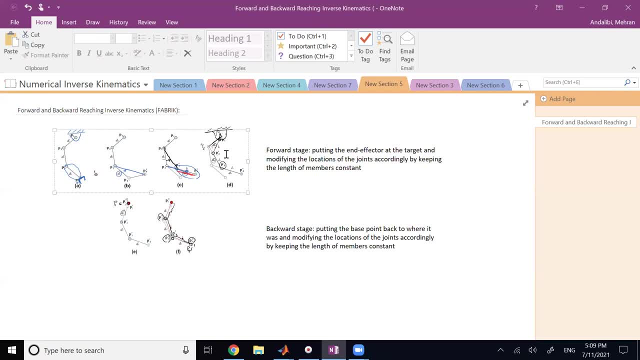 computations. Clearly, you see, the method does not need any calculation of a derivative slope, a divergence, anything like that, a Jacobian, and it's not super susceptible to the initial guess, just like CCD. But of course, again in these, 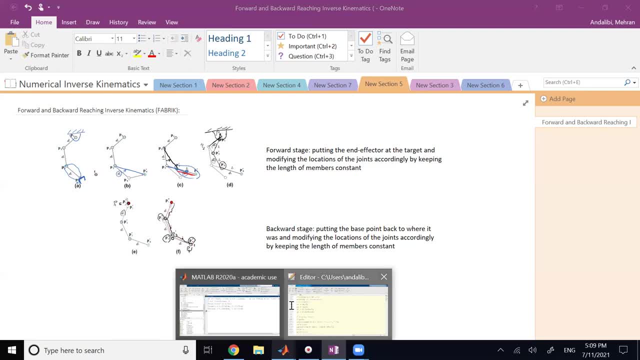 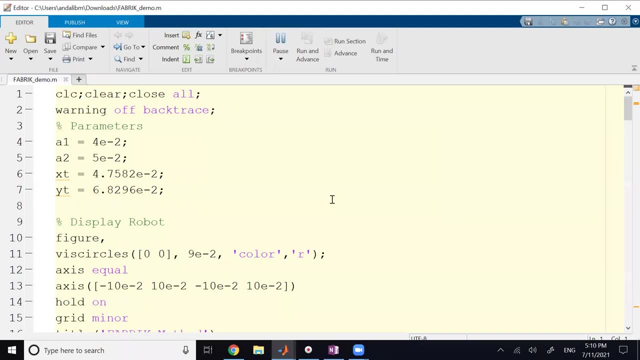 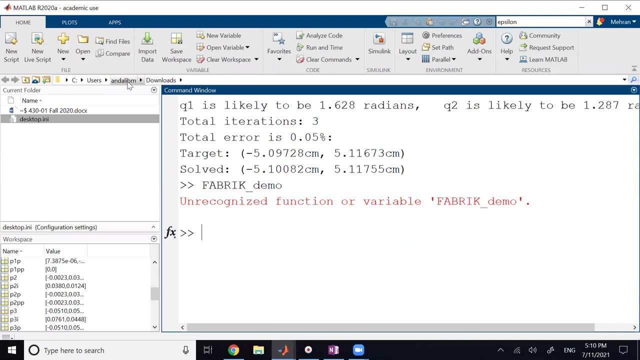 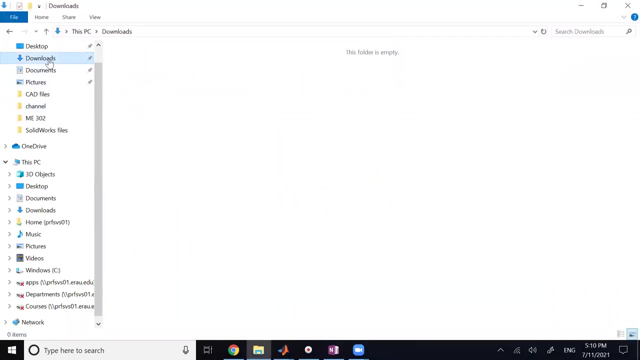 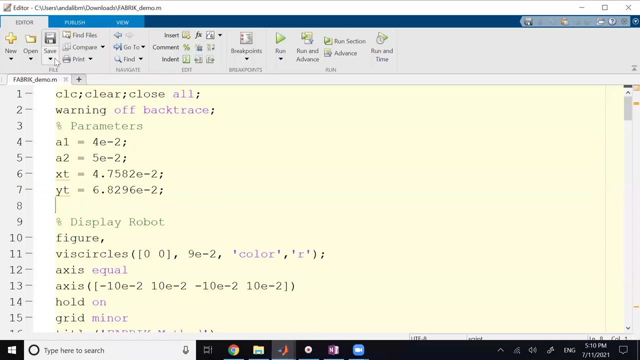 computations. so first let me show you a demo. right, I am going to show you a demo here. Okay, I got some error for some reason. So Okay, Well, that is quite weird, Same as others. One. 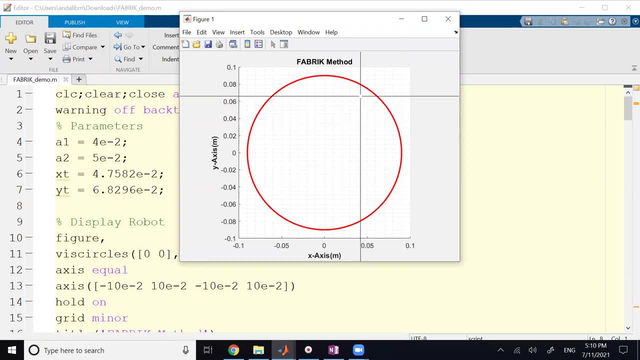 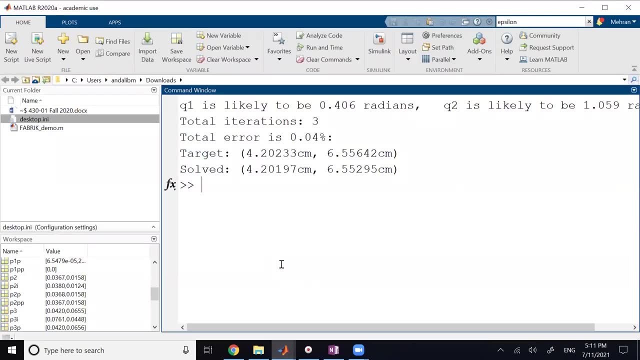 here. Okay. So here I click on some point like this and boom, you see it can get there very fast actually. And you see the error is only 0.04%. It gets you the solution. It only get it three iterations because your target and initial solution were very close. You can see here clearly: 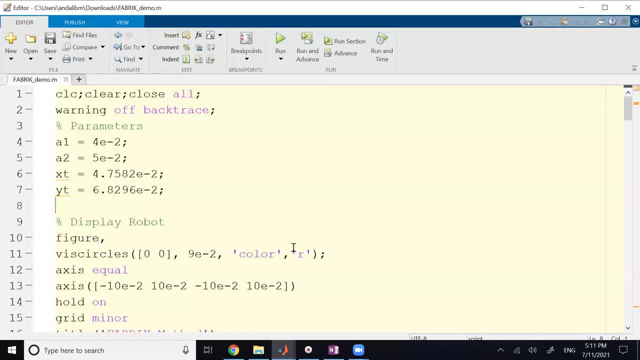 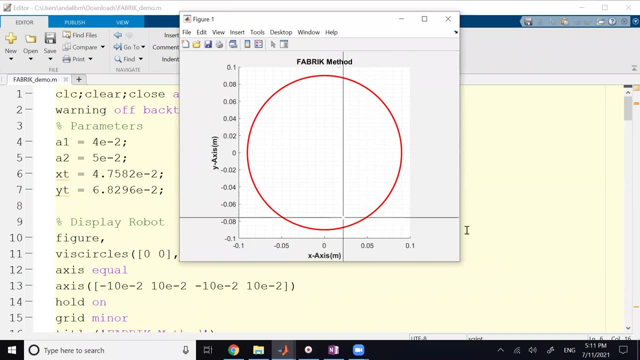 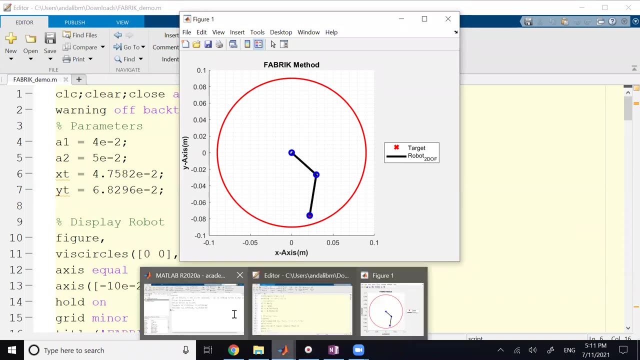 up to two decimals, which is 0.1 of a mil. I have accuracy. Let me do it one more time and try to change my location to somewhere else, maybe here. And you see, it's just a few iterations. That's good enough to see three iterations. You see it's. 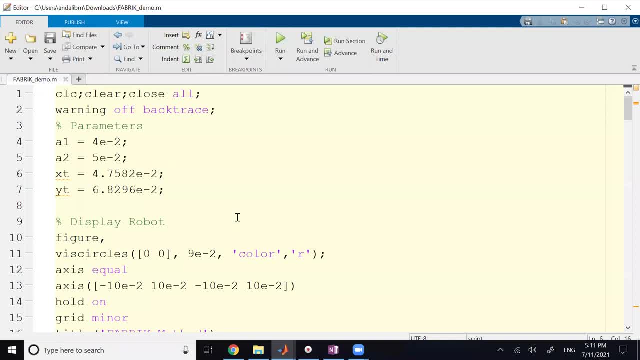 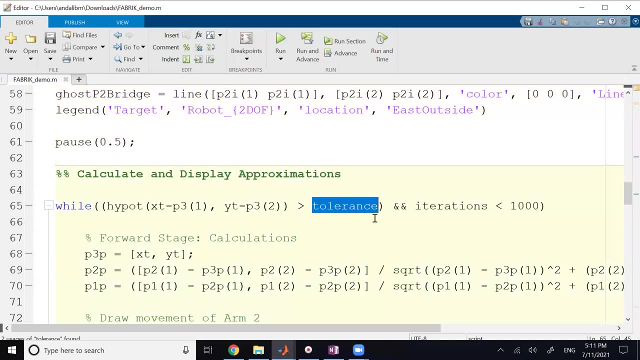 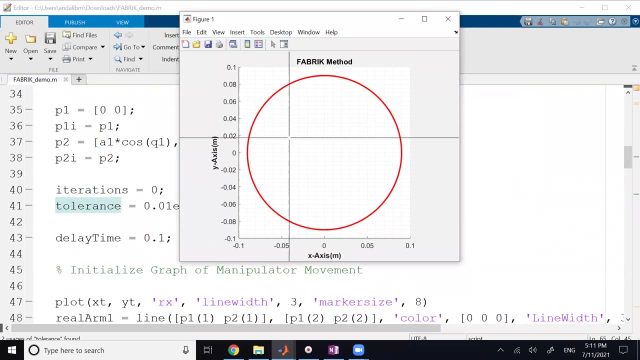 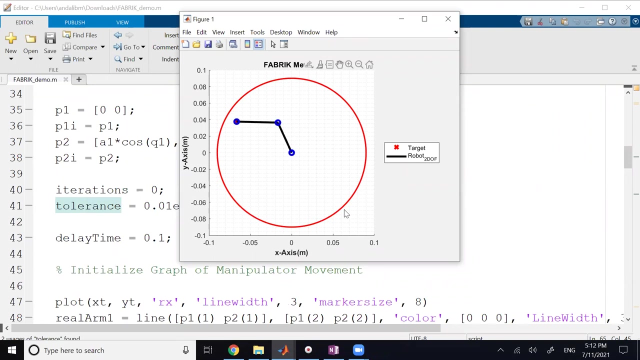 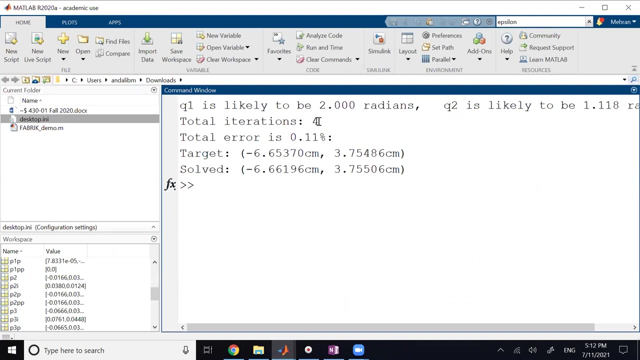 way faster And I guess my tolerance was the same as the CCD method. Let me check that Tolerance. Yes, that's the same tolerance, But you see, this method outperforms the CCD. It's way faster. Look There we go Right Done With a tight tolerance, Easily Four iterations, Of course. 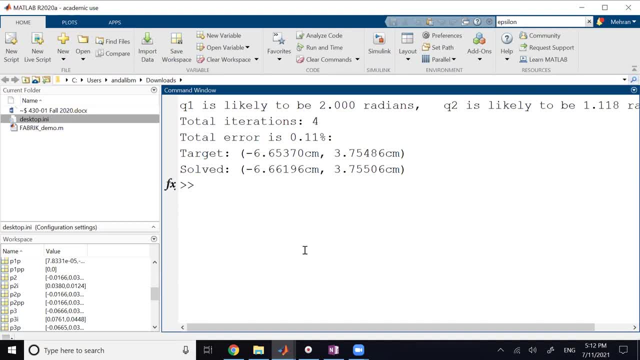 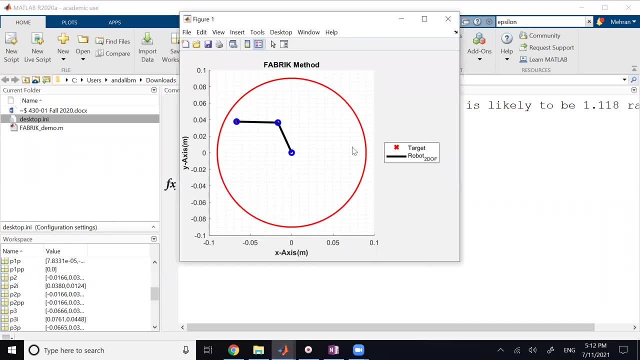 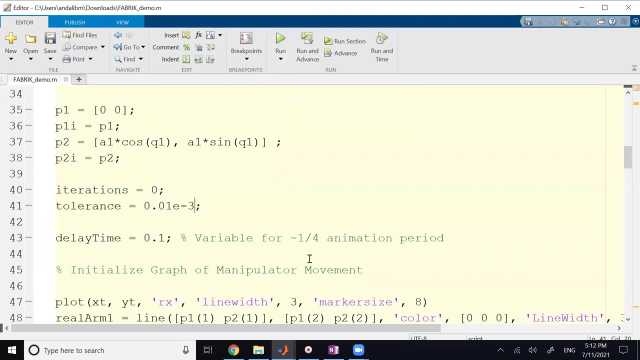 each iteration takes a bunch of computations, but not too much more than CCD really. You see, in terms of tolerance it's way faster and it is not super susceptible to that tolerance. really. Now I might wonder, if I change this to negative three, can it still reach Right? So let's give it some tighter. 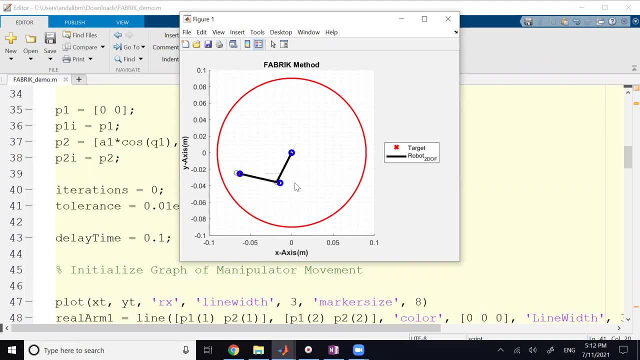 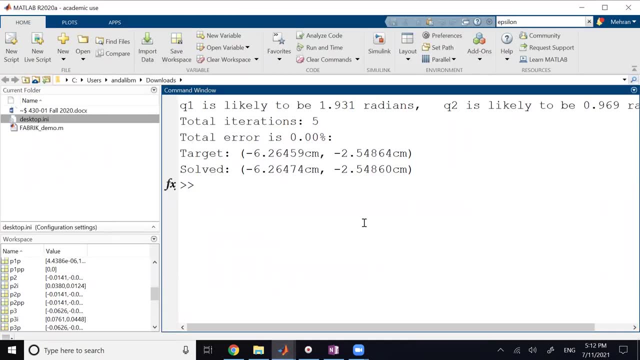 tolerance here. See if it can do. it Seems like it did. Let's see: Yes, Five iterations, And now look Three decimals. So this method is really amazing, right In terms of tolerance. So let's. 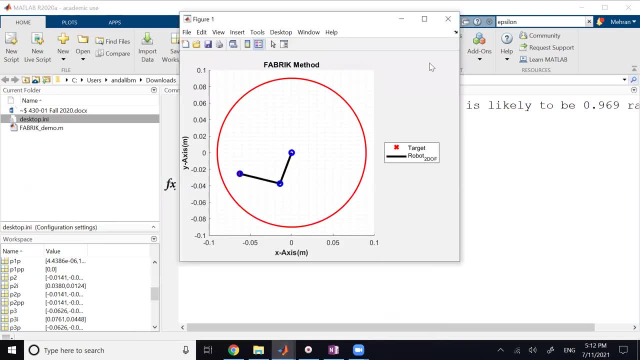 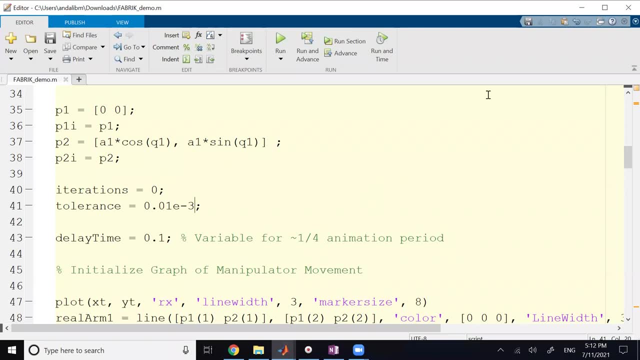 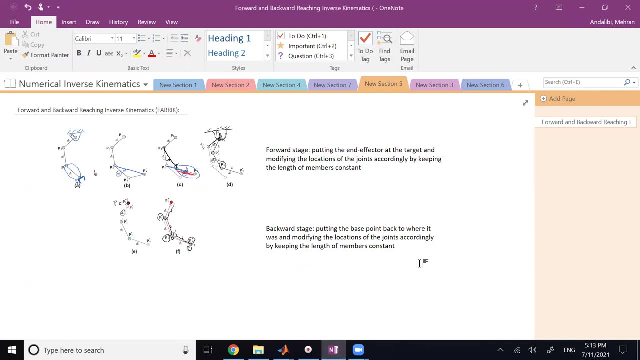 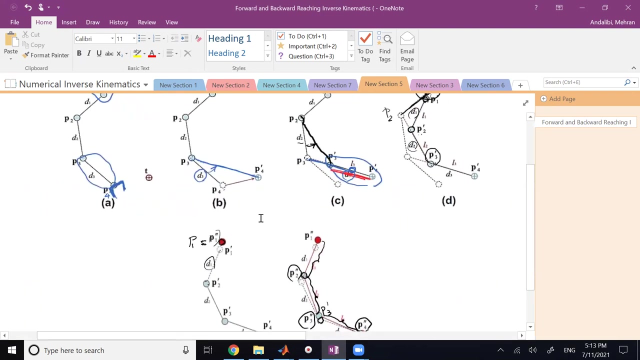 see what it can do, at least for this 2DOF robot. You see, it's amazing. It's very fast, very accurate, And let me just briefly explain the math behind it, Because, again, the math of this method is not super complicated. Okay, So what you do here is this: When I want to update the location, 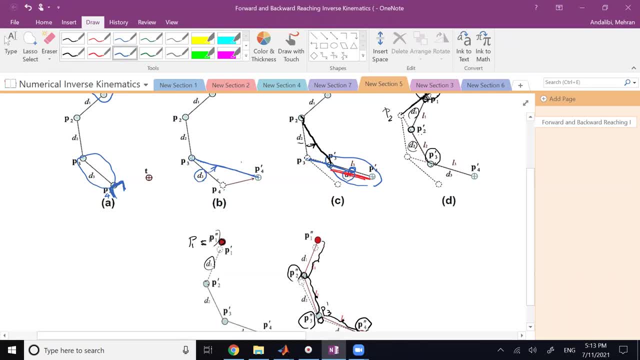 of each joint here. let's say in this first stage: So my P3 goes to P3 prime. So if I have coordinate of P3 and P4 and T and you know, I have all of them, P3 and P4.. P4 is my end effector. 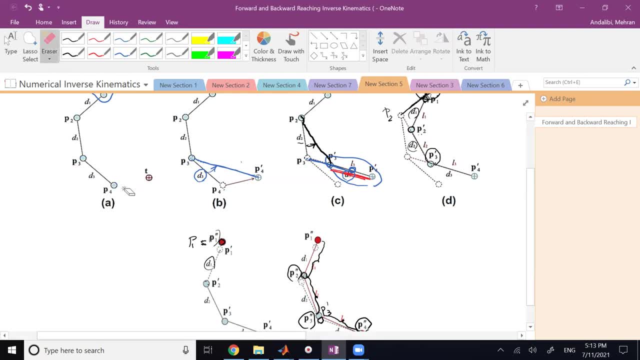 I have all of the joint locations from what From my forward kinematics correct? So I have all of those. So these are all known. at any point, Target is also a fixed location. So the question is: where do I find P3 prime? If I can find P3 prime, that's it. That's all I need Find this location. 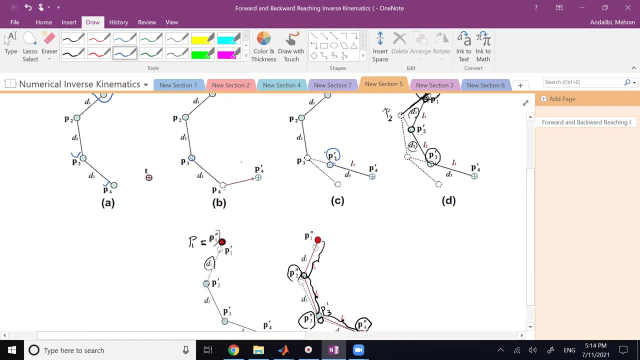 basically, How do I do that? So for that, I need to first get this unit vector which connects your P3 to the target point. I need this unit vector of that line And I choose the direction of it to go. So I'm going to go to the target point And I'm going to go to the target point. 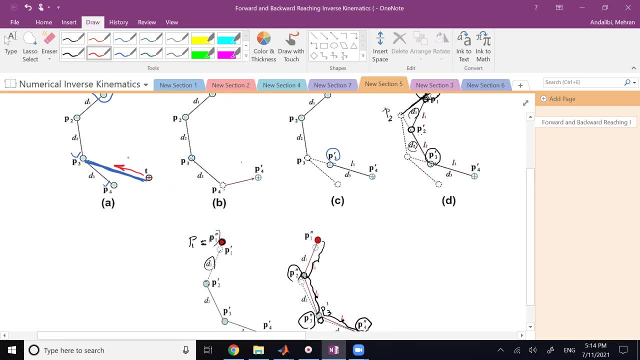 And I'm going to go from target to P3, like this, And I call this U Or, if you want, you can call it U3 and target, If I know the location of the target, which I do, and I know this unit vector. 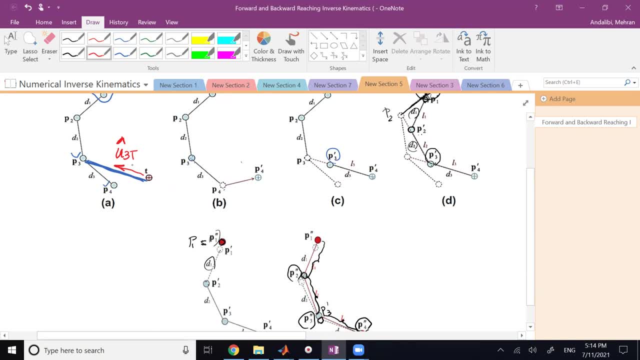 which I can easily find by subtracting T and P3,. if I multiply that unit vector by this distance, D3, that is going to be this vector. And adding that vector to what, To the vector for the target, will give me the vector for P3 prime. 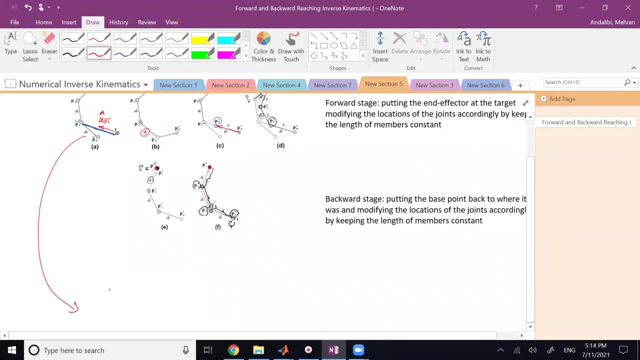 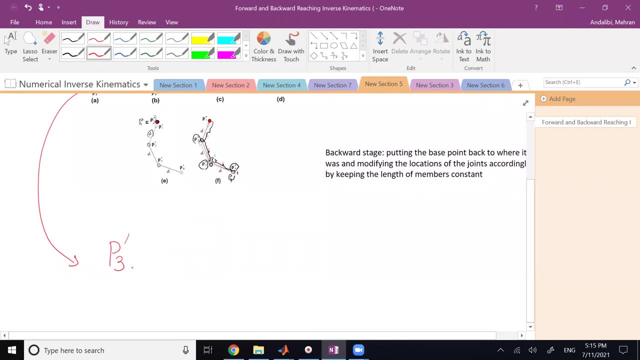 So, as simple as I can say here what That P3 prime right, Which you can call it P3 prime X and Y if you want. This is equal to the target point P of the target X, P of the target Y plus D3, the length of that number times what. 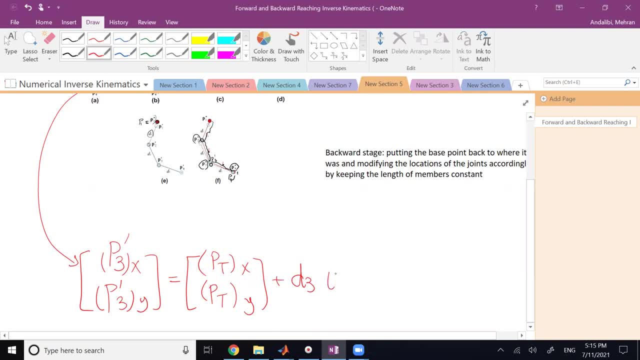 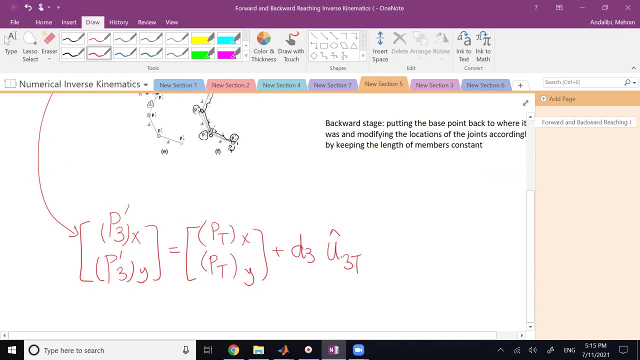 Times the unit vector 3T. And the unit vector 3T, as you know, it is what It is: P of 3X minus P of TX and P of 3Y minus P of TY. This vector divided by, of course, what? The magnitude of it. 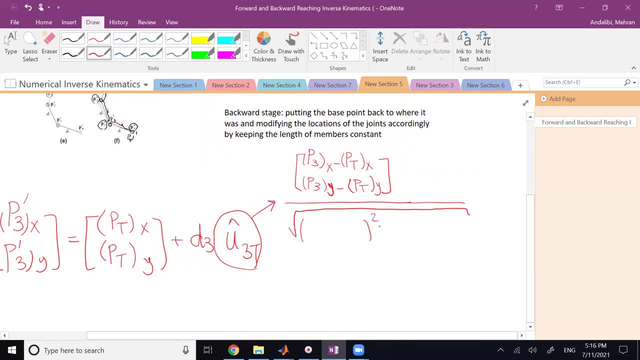 So this vector, divided by, of course, what The magnitude of it? And it is P of T plus T of TX. So, as simple as I can say here what The magnitude of it, And you know again, you have the location of T, you have the location of P3.. 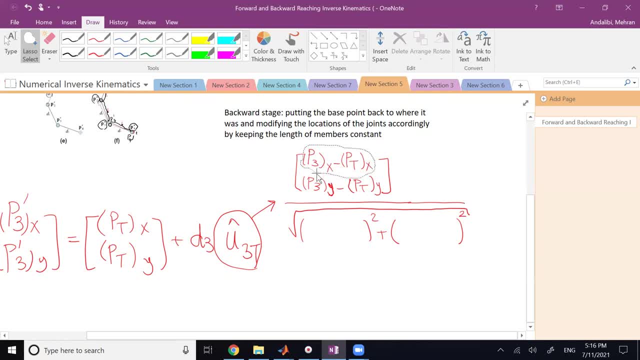 So calculating this should not be any hard thing. Okay, So, as you can clearly see, the math of this method is even easier than the math of the CCD method. It's not any hard math, and that's what I really like about this algorithm. It is easy to implement and you clearly see, in terms 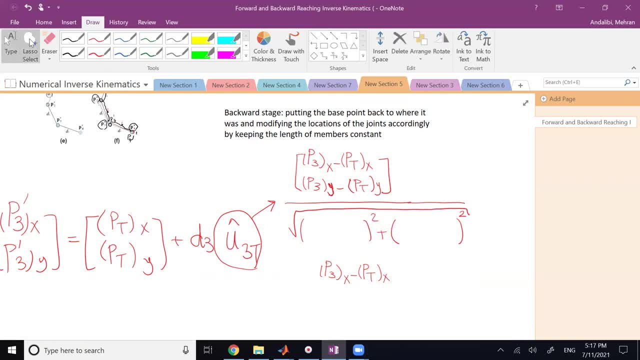 of the power of the method, clearly, clearly outperforms CCD, no doubt about it. Okay, let's see. Let's see if I can get this guy to go here. There we go, And maybe I can get one more of that. 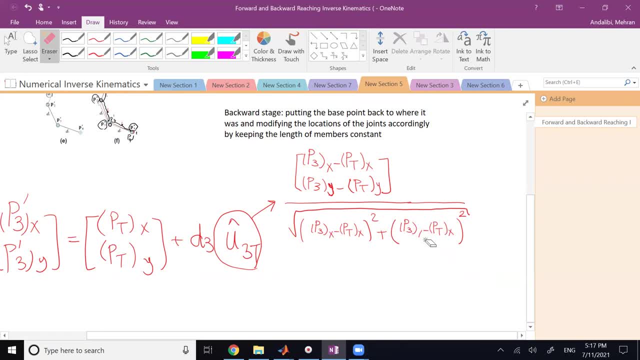 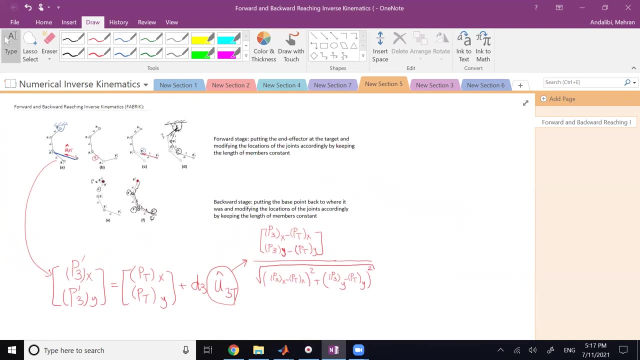 Take it there and then change x to y. It should be easier. But as simple as that, You can get each joint to update its coordinates. You go to the next joint. you go to the next joint, you go to the next joint. This is for forward stage. Now, in the backward stage instead. 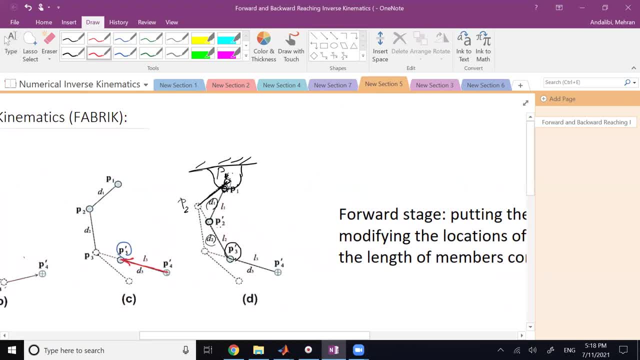 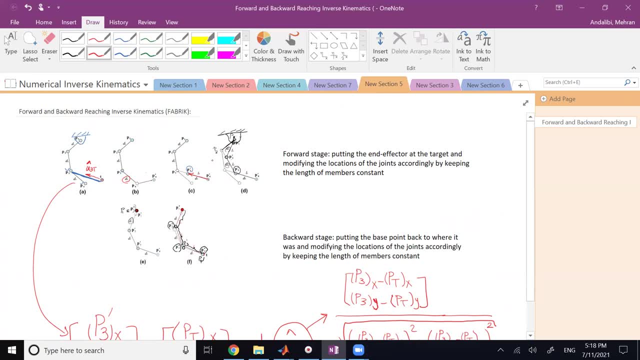 of connecting your points from the last one to the first one to the target, right. So if you see, here I'm connecting each one of my—I connect my last one to the target. Now for the next one. let's talk about that. 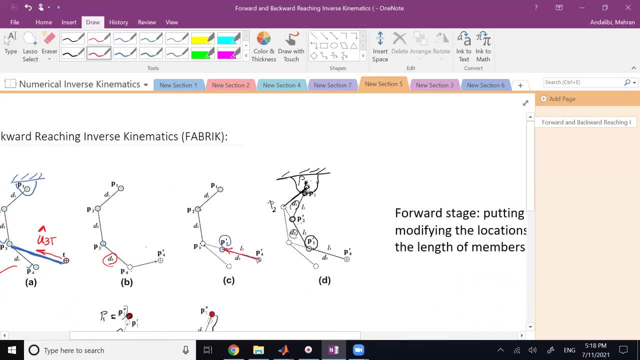 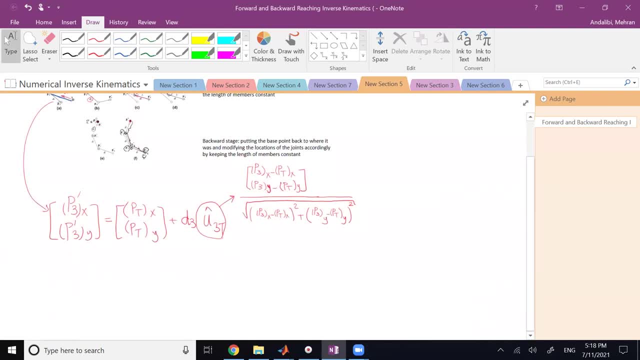 For the next joint P2, I'm not going to connect it to target, I'm going to connect it to what, To joint 3 prime. So for the next one, the update equation is different. It's only for the end. 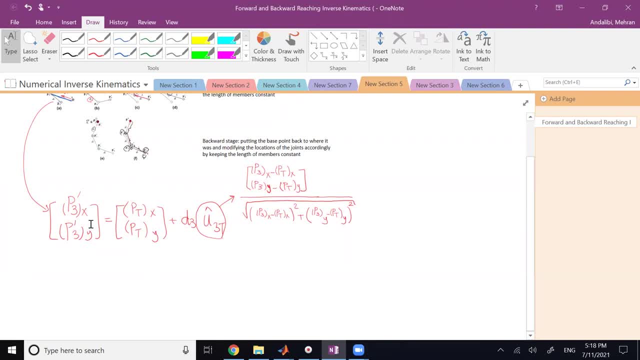 effector one. This is only for the joint right before the end effector. You connect it to the next joint of it, which is then the effector or UT. But for the next one, your update equation is going to be what? 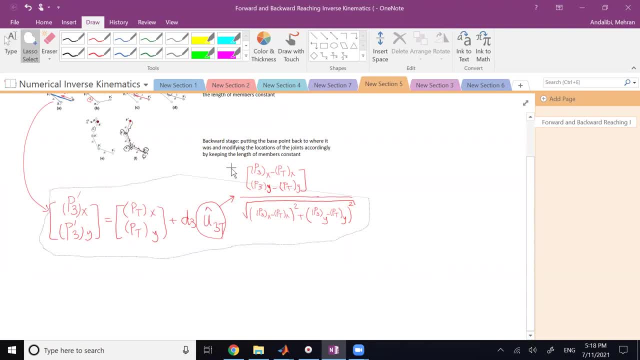 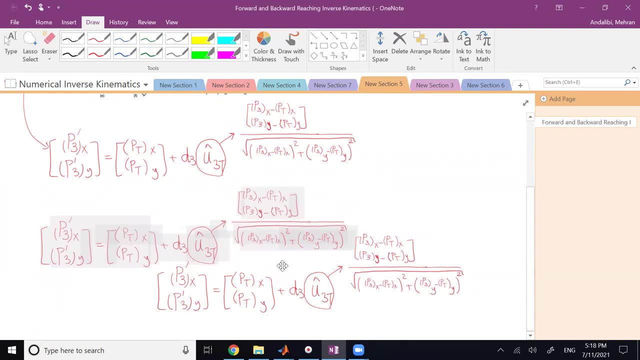 It's going to be a little bit different. So that's your last joint. As I said, for the next joint, where you go to point two instead of three, you're going to need a little bit of change. You have to do a little bit of a change. 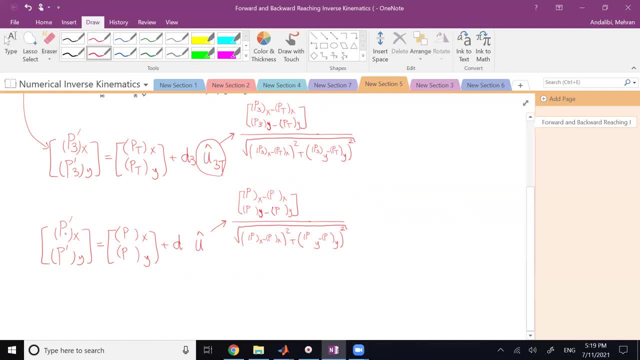 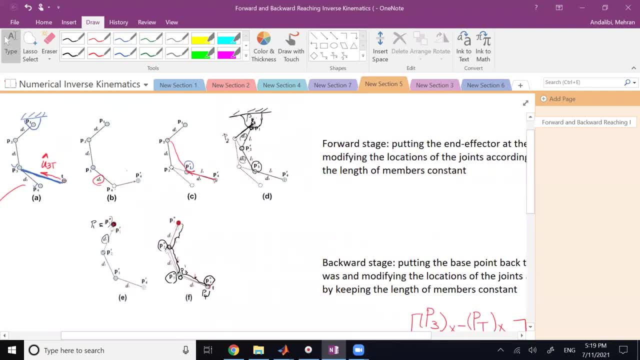 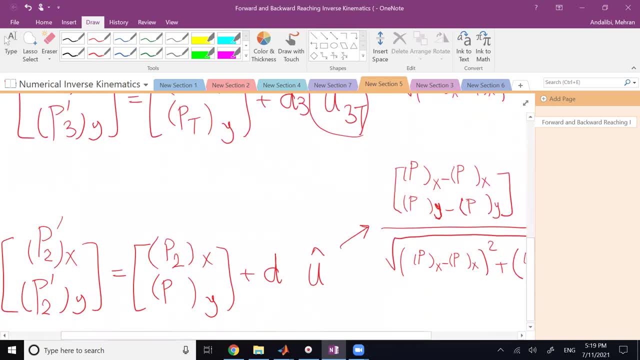 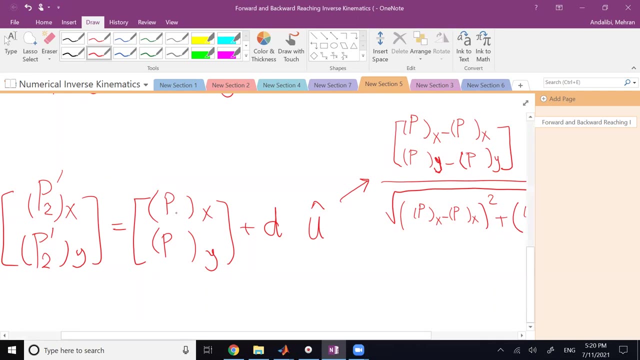 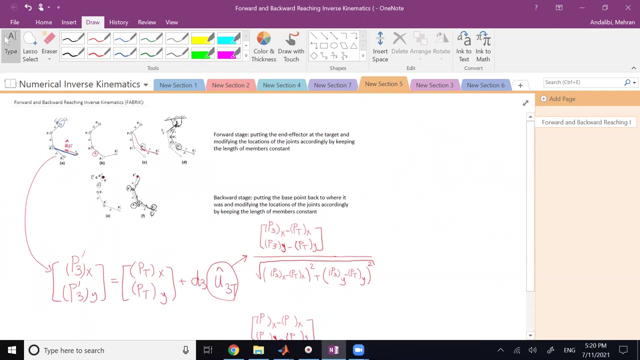 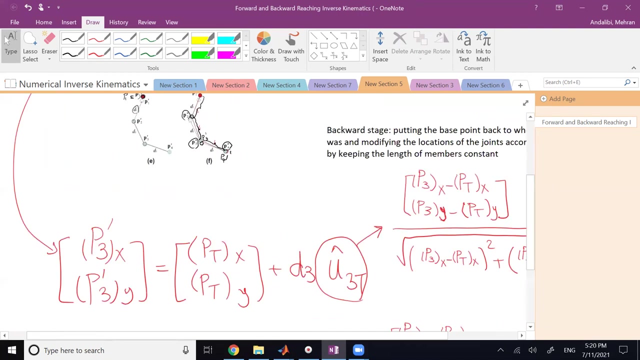 Red telling a coin, Red telling a coin way. P2 is going to be the end of it, which is P3 prime. So this is going to be 3 prime, not 2.. So this is going to be the new location of joint 3, which is 3 prime. You connect it to 2, and then you update it and call it P2 prime. 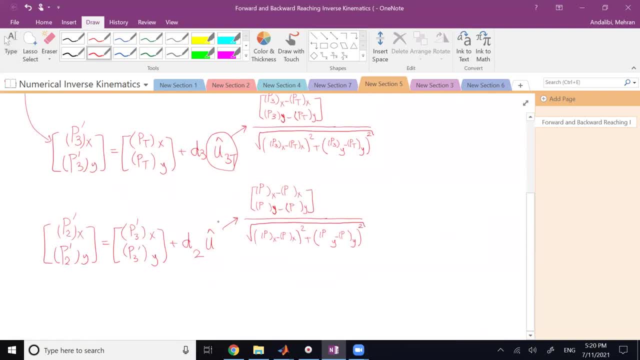 Correct. And then this D is going to be D2, and this U is going to be U of 2, 3.. Which is going to be U of 2, 3.. Correct, And then this D is going to be D2, and this U is going to be U of 2, 3.. 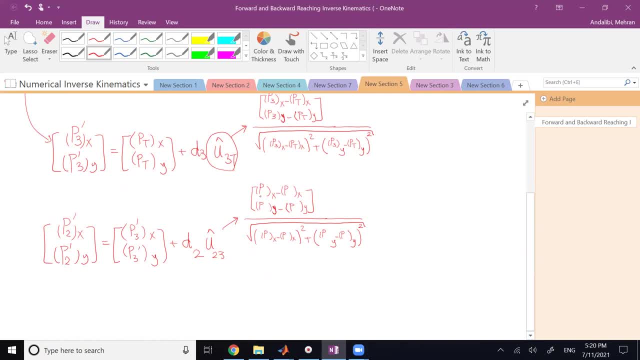 So this is going to be going from 3 prime to 2.. So it is going to be 2 here and it is going to be 3 prime, And then you repeat that Next time it is going to be what? P1 prime. 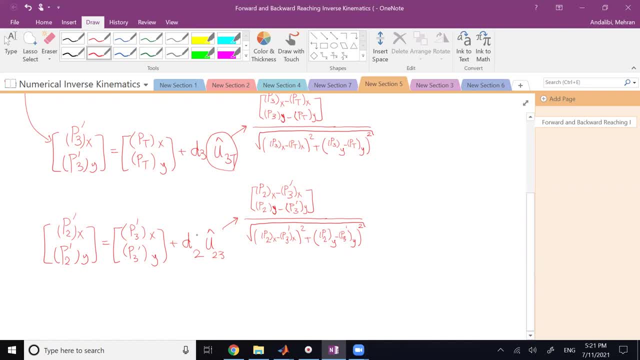 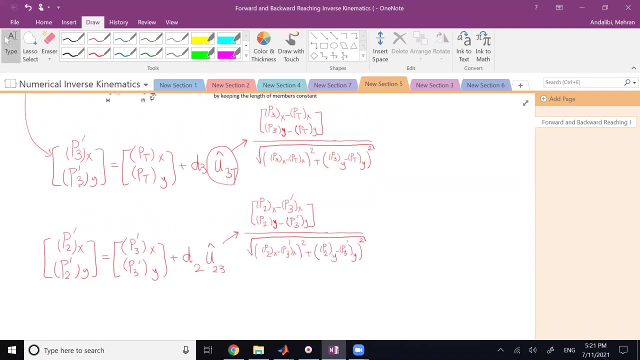 This is going to be P2 prime. This is going to be D1.. This is going to be U1, 2.. So it has P1 in it and P2 prime that you got from this stage Right. So you see the number that you get for P3 prime. you need it here. 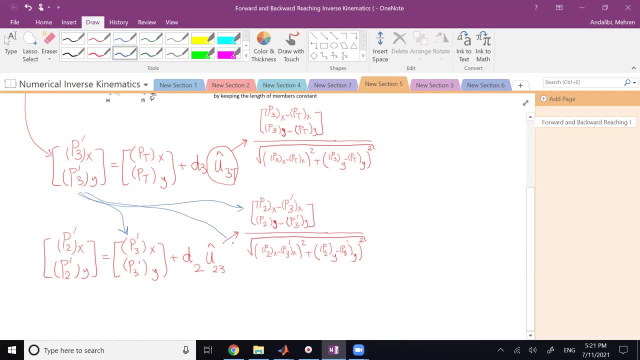 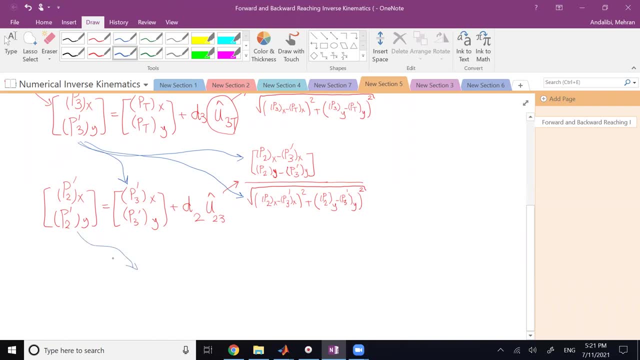 And you need it in those guys over there. And, as I said, when you go to the next stage for P1 prime, you need this P2 prime, You need this P2 prime. X and Y, Correct. And then you repeat that. 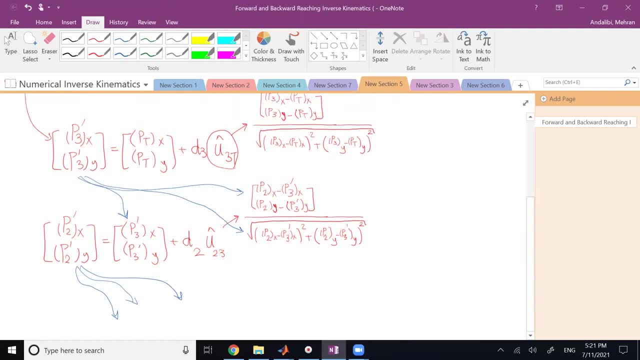 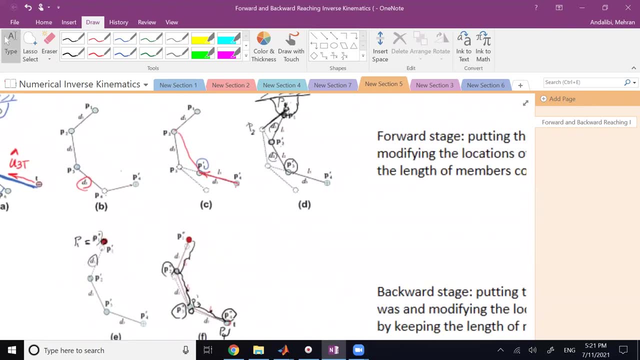 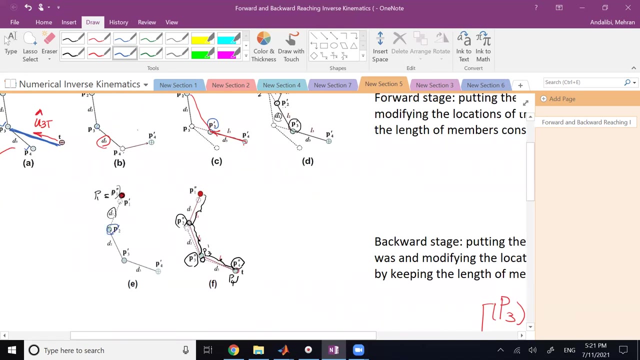 So it is in stages, The data you get from each iteration. you need it in each calculation, You need it in the next calculation. So you go all the way like this until you are forward, The stage is done. Now, when you go backward the stage what happens is for the first joint that is right next to the base. 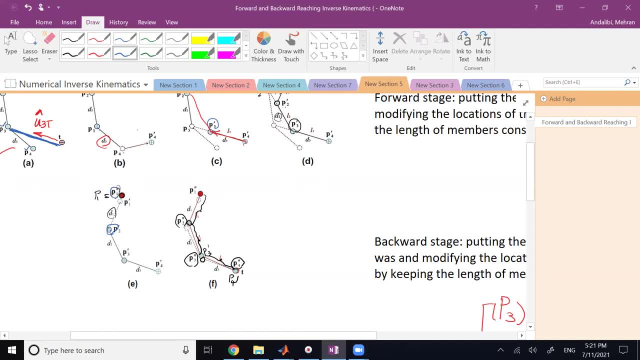 you put this P1 double prime to be the same as original. Original, as I said, location of P, which maybe you can call it, for example, 0,, 0 or whatever you want to call it, And then again updates, Right.